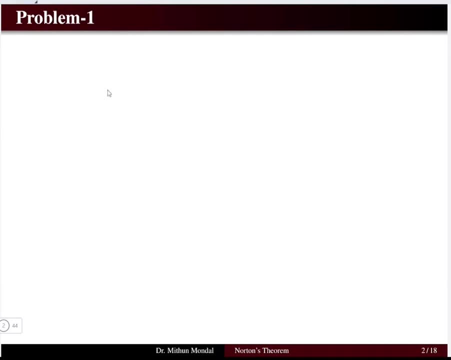 theorem. So little bit overview of the Norton's theorem let us see, so that how you will be solving the problem you will able to know that. So what does Norton's theorem suggest If you have any complex circuit? complex circuit means a circuit which is having 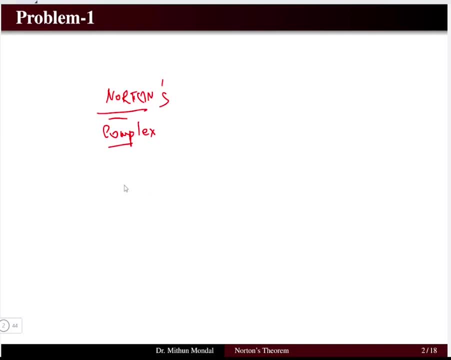 too many sources or the passive elements, like that, then in that case you can reduce the circuit into a simple equivalent circuit consisting of a current source, which is known as the Norton current, in parallel with a resistance which is known as the Norton resistance, R Norton. So what is the Norton resistance? So what is the Norton resistance? So what is the Norton resistance? 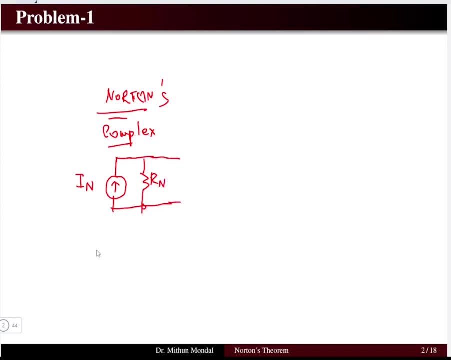 So what is the Norton current and what is the Norton resistance that you have to calculate? Norton resistance is simply the Thevenin resistance that we have calculated when we have studied the Thevenin's theorem. So Norton resistance and Thevenin's resistance are same thing. 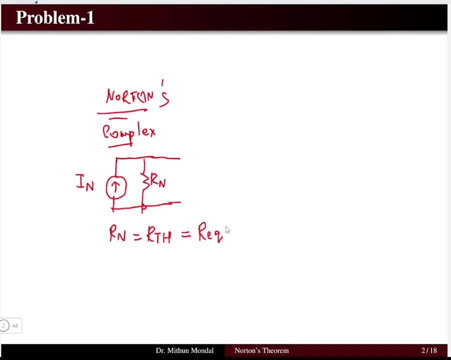 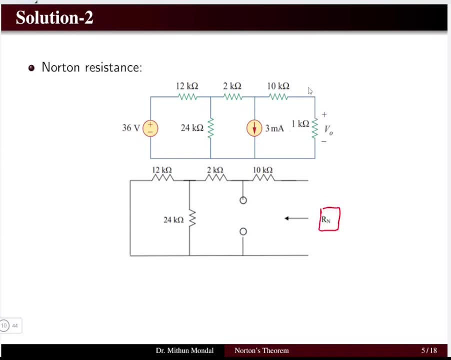 resistance when the terminal is open circuit. So Norton resistance and Thevenin resistance are the equivalent resistance when the loading resistance are nine- 10.. So we have to remember resistance when the loading resistance are nine- 10.. So we have to remember the variable resistance. 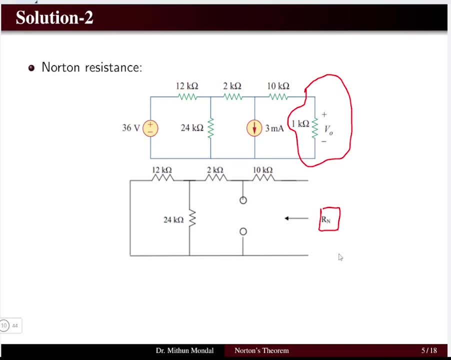 or the load resistance from the network. So first, So you remove load resistance with an open circuit and towards the terminal, inside the terminal. You have to see it. you have to see it how you disconnect the independent sources. So we have a 36 Volt independent. this 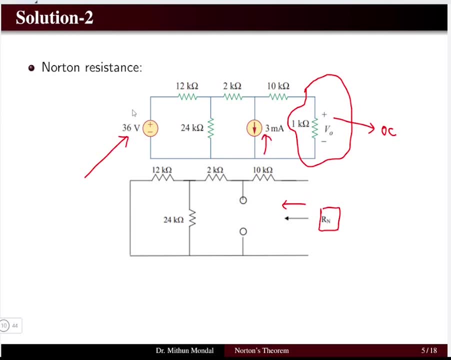 And 3 mA current source independence. So voltage source will take agent and so current source is be replaced with a short circuit. Current source will be replaced with open circuit. So we have short circuited the voltage source and open circuited the current source. Now we are in. 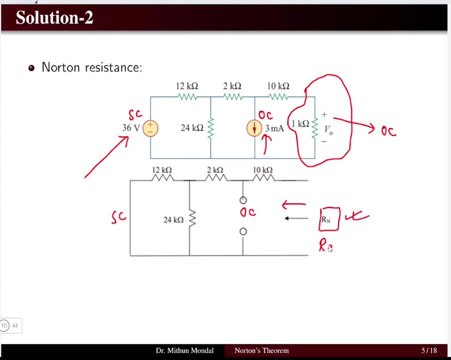 a position to determine the R0, which is basically the equivalent resistance. So if we see this circuit, we find that 12 kilo ohms and 24 kilo ohms are in parallel and that is in series with 2 kilo ohm and then it is in series with 10 kilo ohm. So we can apply the series parallel concept. 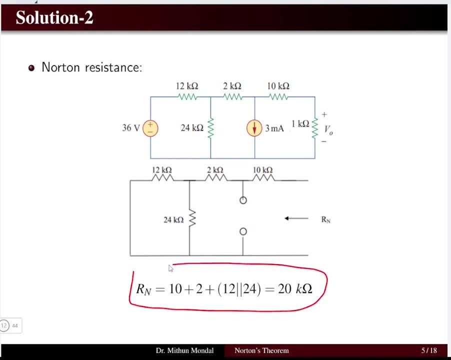 that we have studied to find the value of R0. So R0 is basically the equivalent resistance, that is, 20 kilo ohms. This is similar to R Thevenin, which we have calculated in the Thevenin's theorem. So 20 kilo ohm is the value of R0.. Now we have to obtain the I0. So in order to obtain the, 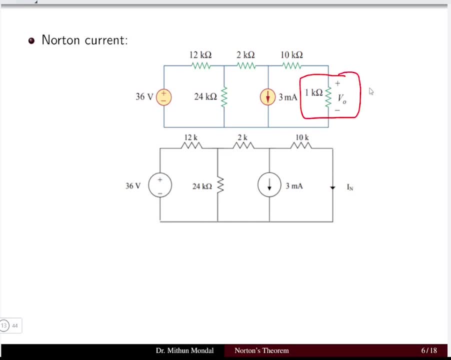 I0,, we have to obtain the I0.. So, in order to obtain the I0, we have to obtain the I0.. In the I0, the load register is short circuited. So RL, which is the load register, is basically. 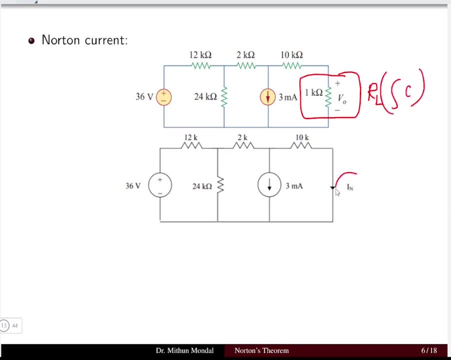 short circuited. So we have the short circuit current which is flowing here, that is known as the Norton current, that we need to determine, Keeping the other part of the circuit as it is. So we have a 36 volt source and 3 milliampere current source and other resistances we have 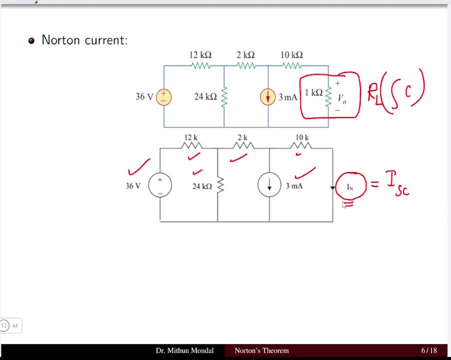 So we have to determine the value of I0.. The value of I0 is the value of I0.. So we have to determine the value of I0.. The value of I0, that is the short circuit current, we can determine by different techniques. 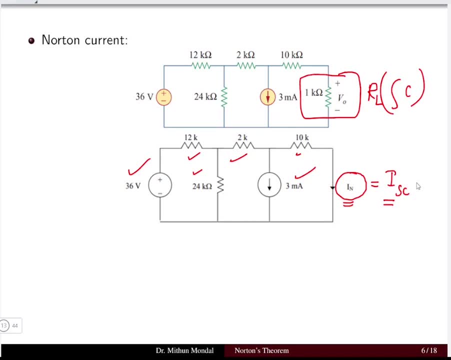 whether it is a KVL, KCL, superposition, source transformation, any theorem we can apply it. Now, if we apply superposition theorem, then let us see how to find the value of I0.. So superposition theorem: we have studied in the lecture class that. 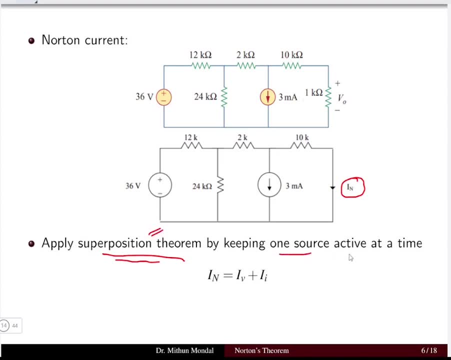 superposition theorem will have one source which is active at a time. So we have a voltage source and we have to find the value of I0.. So we have to find the value of I0.. So we have to find the value of I0. 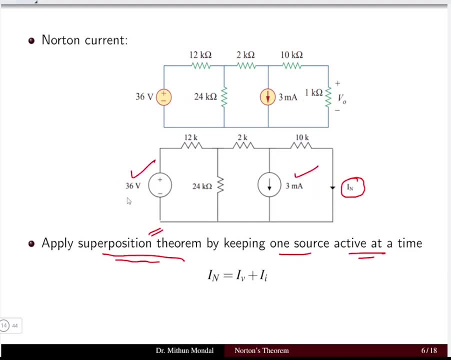 So we have a current source and one source you keep active at a time and then you determine the corresponding response at the terminal, which is the load terminal. So you can find the Norton current as the sum of all the responses due to individual source. So you have IB. that is the. 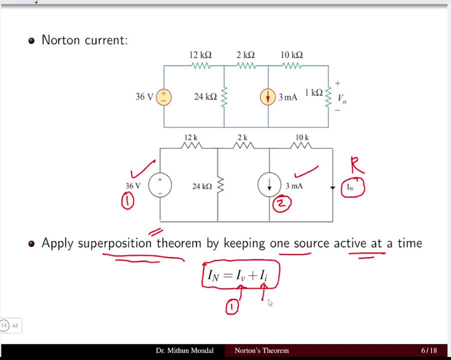 current at the terminal due to source 1, and II is the response due to the source 2.. So we have a voltage source and we have a current source. We will keep one source active at a time. So when we keep the voltage source active, then the current source will be open circuited. 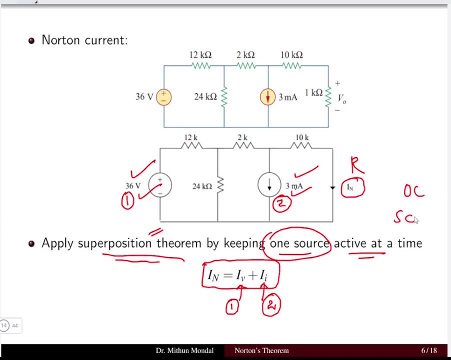 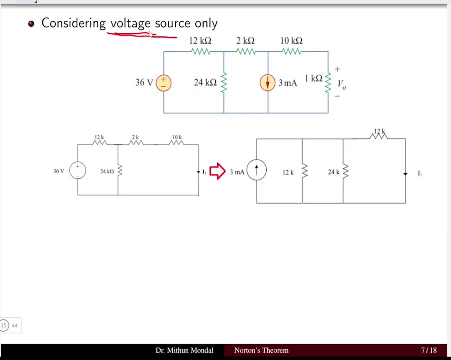 When we keep the current source active, then the voltage source will be short circuited. So let us see how to do this Now. you keep the voltage source active at a time, So we have a 36 volt and 3 milliampere. I will keep the 36 volt active, So it means that 3 milliampere has to be. 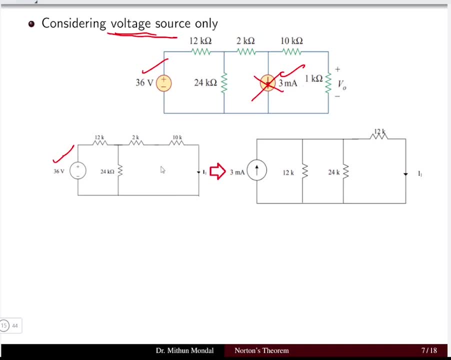 removed from the network, which is removed using the open circuit. So we can open circuit these two terminal of the current source and then we can determine the value of the current which is flowing at the load terminal which is written as I1.. Now these again can be calculated: I1 can. 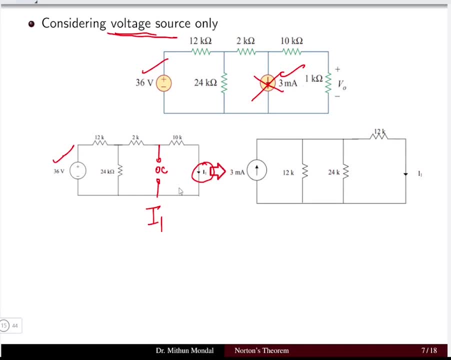 be calculated using KVL, KCL or other techniques. Let us apply the source transformation here. Okay, Okay, If we apply the source transformation. so in this particular problem we will be studying the Norton's theorem, the superposition and the source transformation. All are combined in this. 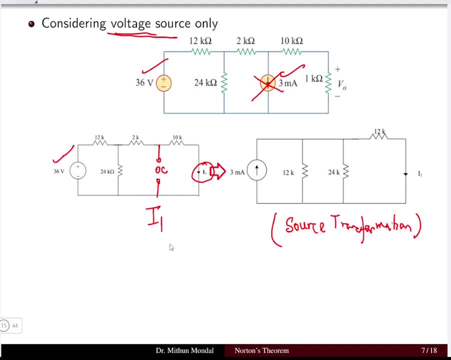 particular problem. So source transformation: if we apply, then we see that 36 volt and 12 kilo ohm resistor can be replaced with a current source in parallel with a resistance, where the current source is basically voltage by resistance. So we have 36 volt. 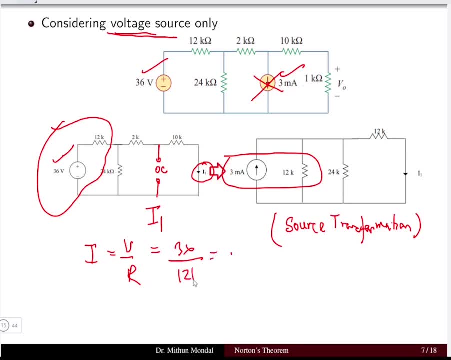 divided by 12 kilo ohms, which will be given, giving us 3 milliampere as the current and the resistance is 12 kilo ohm, which is coming in parallel. Now it is very easy because we have series, parallel combinations, like these two registers are in parallel and which is in series. 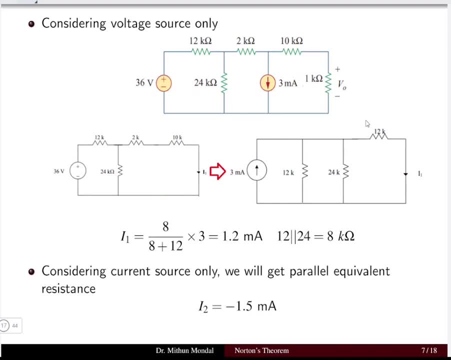 with a 12 kilo ohm resistor. So we can do that to find the value of the current. Okay, So what we can do is that we can find the current. So we can do that by finding the value of the current. 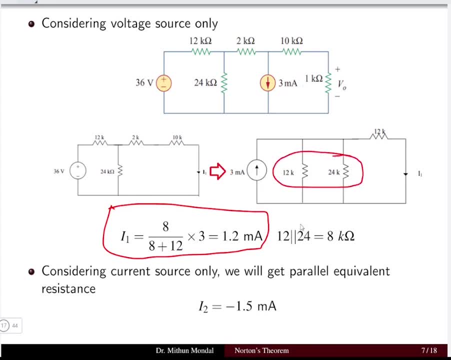 find the equivalent resistance of these two network, or the resistance which is equal to 8 kilo ohms. Now our circuit will be like this: We will be having a 3 milliampere current source, one resistance which is of 8 kilo ohms, which is the parallel combination of 12 and 24. 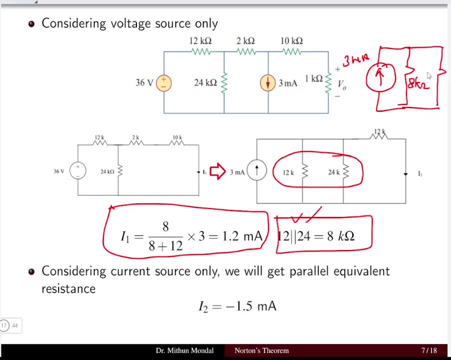 and then we have a resistance which is equal to 12 kilo ohm. right Now we have to determine what is the current I1 flowing here? It means the same current will be flowing here also, that is, through the 12 kilo ohm resistor. So we can apply the current division rule. Now you see how we are. 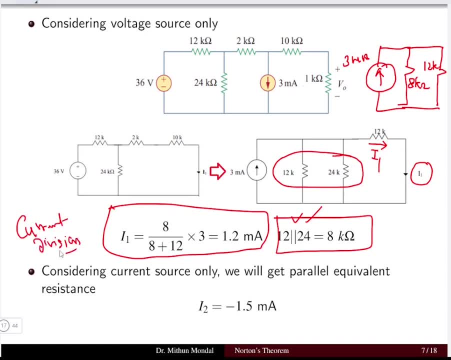 moving from one theorem to another. We have started from Norton's theorem, then moved to the superposition, then source transformation and now the current division. So using the current division rule, we can find what is the current which is flowing here, that is, the source current which. 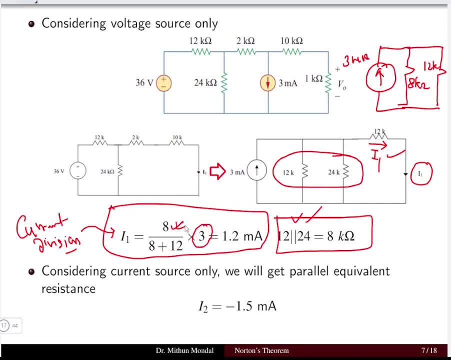 is 3 milliampere multiplied by the current division. So we can apply the current division rule with the numerator. you will have the resistance which is in parallel, that is, 8 kilo ohm, divided by the sum of the resistance, that is 8 plus 12.. We will get 1.2 milliampere as the current, which is 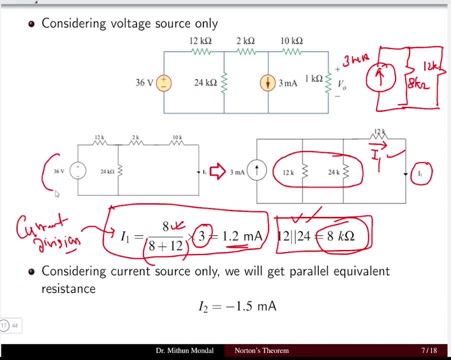 flowing when only one source, that is 36 volt, is acting. So from the superposition theorem we have find out- my first case- that I1 is equal to 1.2 milliampere. Now my second case will be: there is a current which is flowing here, So I will keep the current source active and the voltage source. 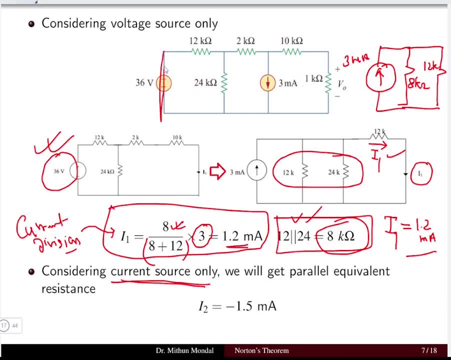 will be removed. So if the voltage source is removed, I will be removing this with a short circuit and I will keep this current source active and I will try to determine the value of the current. that is sorted here. What is the current I2 that is flowing Now? this is in accordance with. 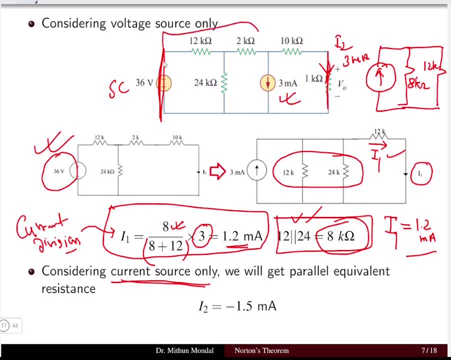 superposition theorem. So we see this left part of the circuit and right part of the circuit. We can do the series parallel combination of the current source and the current source. So we can see that this current source is in parallel with the current source and we will have a simple. 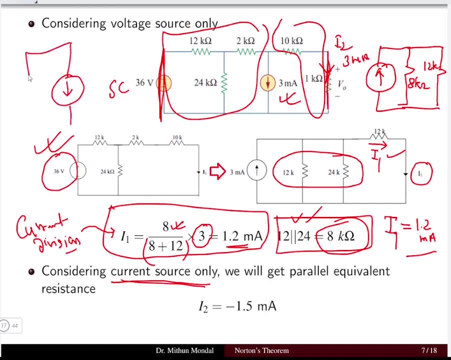 circuit where we will be having a current source, one resistance this side and one resistance this side, and we will be able to find what is the current I2 which is flowing here. So this is with the series parallel resistance. So current I2 that we will be getting is minus 1.5 milliampere. 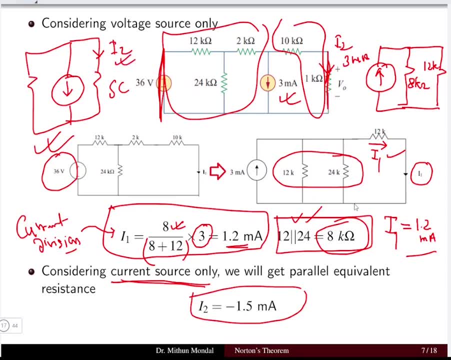 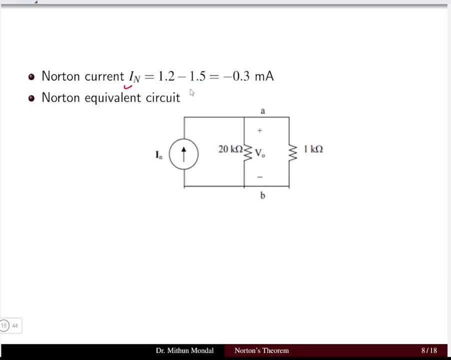 This current which is flowing minus 1.5 milliampere. So we have two currents due to the two sources of superposition. So we have two currents which are in parallel. So we have two position. then we can find the Norton current by adding the two currents, which gives to be minus. 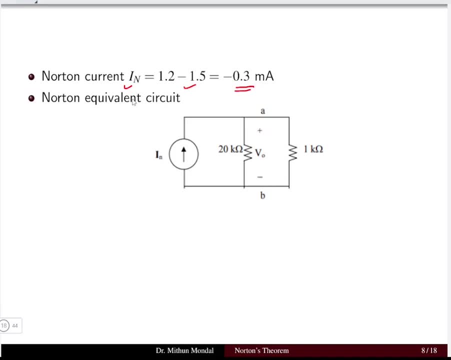 0.3 milliampere. Now the Norton equivalent circuit is basically a Norton current in parallel with a resistance that is R Norton. Now the variable resistance, which is the load resistance, will be reconnected to the equivalent circuit which is obtained from the Norton theorem. So I Norton. 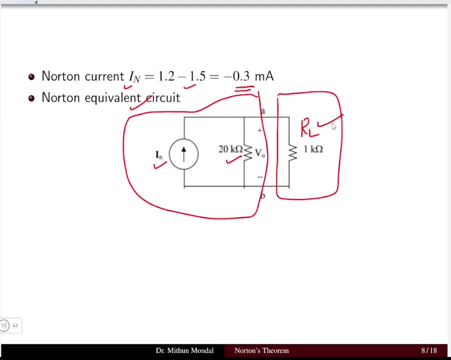 and R Norton we have obtained and the value of R L that we have removed. now we will be reconnecting. that is 1 kilo ohm. Now it will be easy to determine the potential which is across the 1 kilo ohm resistor, which is nothing but the voltage across this. So if we apply the current 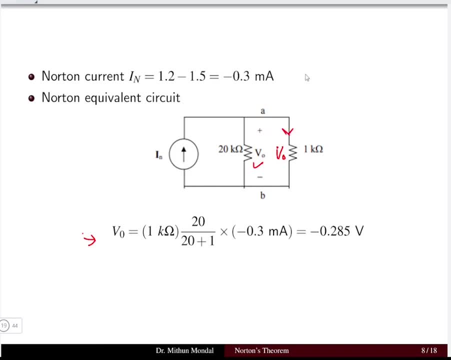 division rule and try to determine what is the current which is flowing here. I take this current to be I x. So I x is the current which is equal to I Norton Multiplied with the parallel resistor. that is, 20 kilo ohm divided by 20 plus 1. that is the 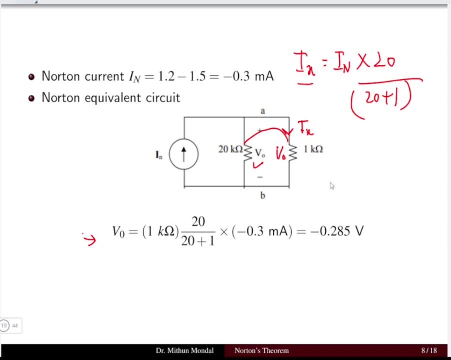 equivalent resistance. So I will find what is the value of I x. Now the voltage V naught that we need to determine is basically I x, that is the current multiplied with the resistance, that is 1 kilo ohm, and that we need to determine. So here we will be, getting the voltage as 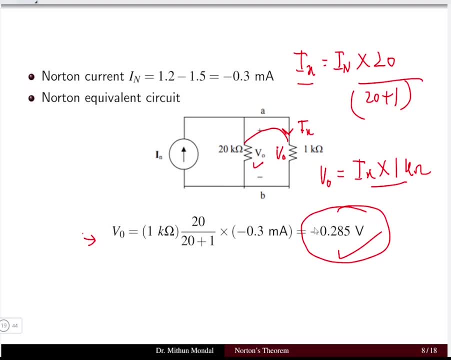 minus of 0.285, where minus sign just simply means that the polarity will be reverse for what we have seen. So this problem is solved. Problem number two, where we have applied the Norton's theorem, superposition, theorem, source transformation, current division, voltage division rule. So this problem covers many concepts at a 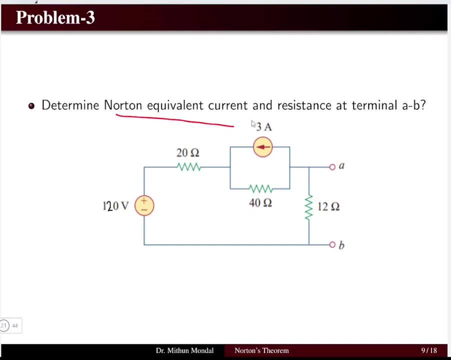 time. Problem three: you have to determine the Norton equivalent current and resistance at terminal A, B. So you have a source 120 volt and there is a source of 3 ampere. both are independent voltage and resistance. So you have to determine the Norton equivalent current and. 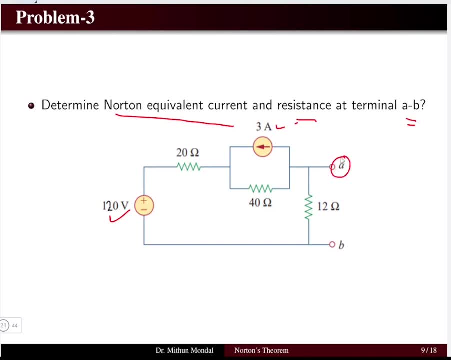 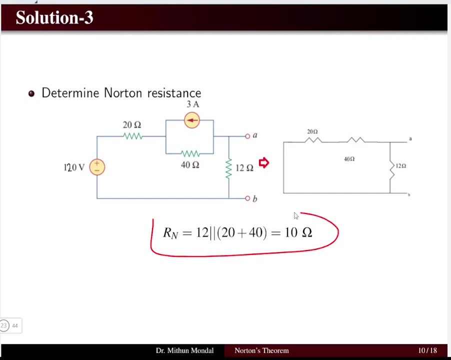 independent current source. Let us try to determine the Norton current and Norton resistance at the terminal A, B. So what we do? first we find the Norton resistance, So short circuit, the voltage source, open circuit, the current source, and redraw the circuit into its format to obtain the R Norton. 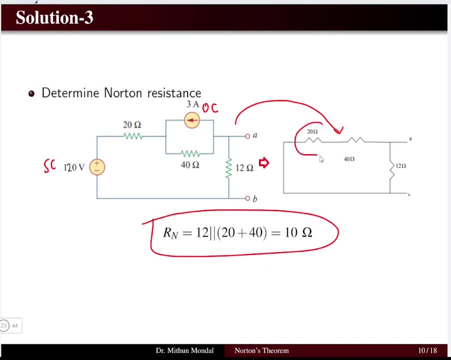 So what we can find? that the 20 ohm resistor and 40 ohm resistor are in series, which is in parallel with 12 ohm resistor, So you will get 10 ohm resistor and 20 ohm resistor are in series. So 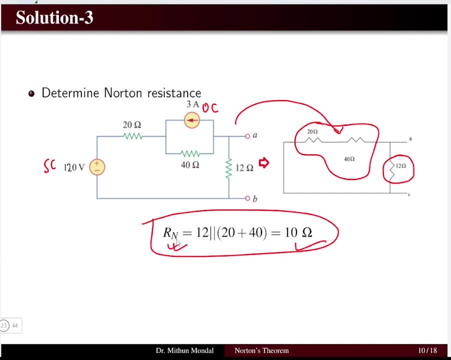 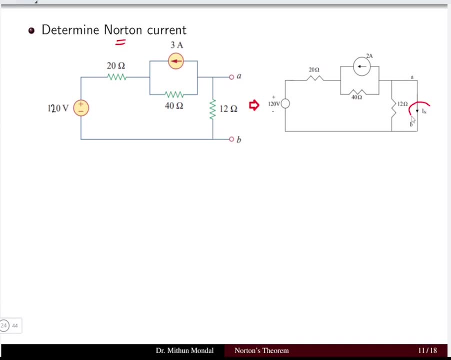 this is what we have found out. Now we determine the Norton current. So to determine the Norton current, we short circuit the terminal A B. So you short circuit the terminal A B of the original circuit. that will be the Norton current which is flowing Now you can apply different theorems. 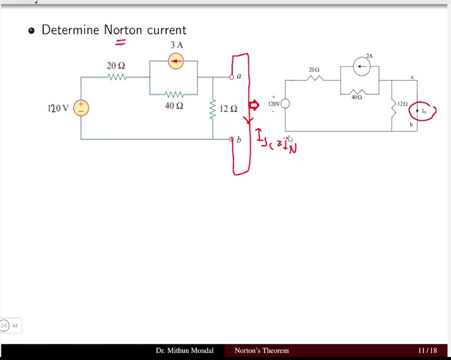 KVL, KCL as superposition, source transformation, any theorem you can apply to find the Norton current. Let us see how to do that. I will be applying the source transformation So these part of the network I can reduce into a simpler format, that is, we can have a voltage source in series with a resistance, So voltage 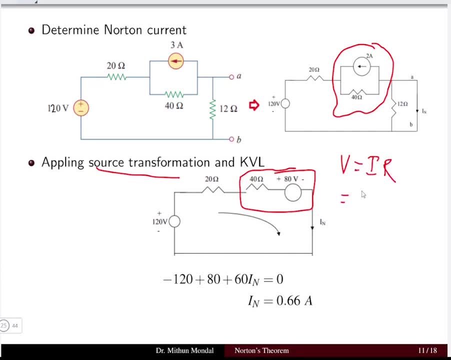 source is nothing but current multiplied with resistance. So we have 2 into 40. that will be equal to 80 volt. 80 volt will be in series with 40 ohm. So here we have applied source transformation. Now we have only one network. 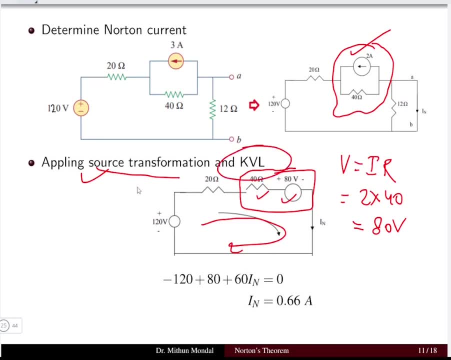 We can apply the voltage law or the mass analysis to determine the value of the Norton current. So you apply the KVL, that is algebraic sum of all the voltages in a closed loop is 0. You will be getting the Norton current as 0.66 ampere. So we have obtained the value of Norton current and the. 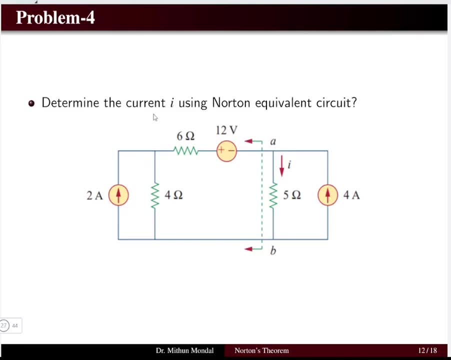 Norton resistance. Problem 4: determine the current using the Norton equivalent circuit. So you see which is flowing through 5 ohm register. So wherever you need to determine the variable, that will be your load terminal, RL. Okay, So you will be having A and B as the load terminal that you need to. 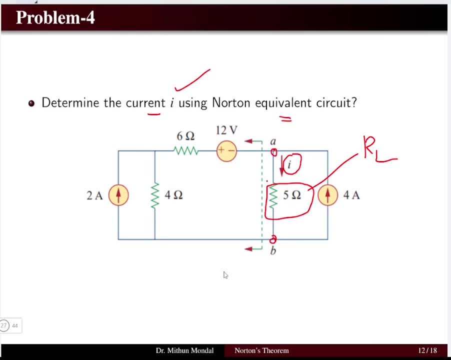 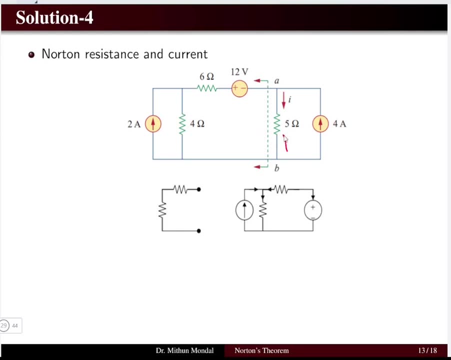 remove from the circuit and determine the Norton resistance and Norton current. So let us see how to do that. Once we remove this 5 ohm register, which is basically a load register, and then we disconnect the Norton circuit. So what we are getting is independent sources, that is, we will be short. 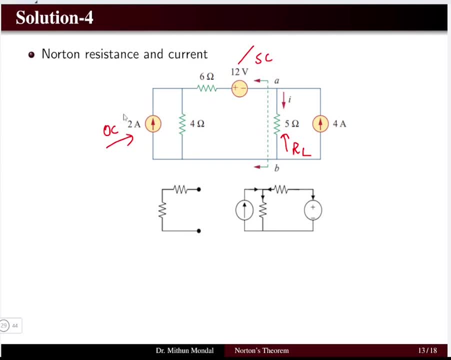 circuiting the voltage source and open circuiting the current source What we are getting. So if we open circuit this, this will be removed from the network. This will be short circuited. Then these parties open circuited. So this part is open circuited because we need to find the value of the. 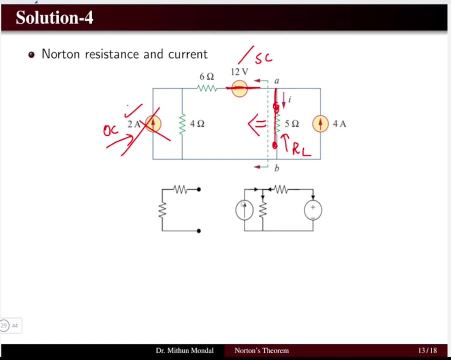 resistance, Okay, And we have to see the circuit from this end like this: Okay. So if we are seeing this end to find the R Norton, we have 6 ohm and 4 ohm which are in series to each other. This 6 ohm- 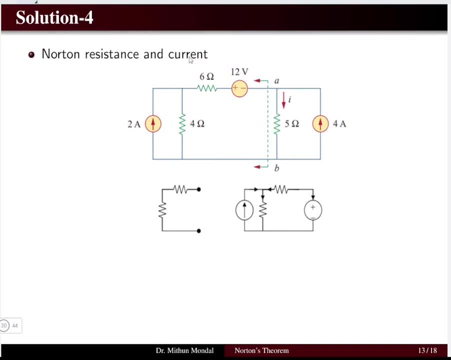 and 4 ohm will be in series, So we will be able to determine the R Norton as 6 plus 4, that is 10 ohms. So you have a 6 and 4 and that combination will give 10 ohms as the R Norton. Now, if I need to, 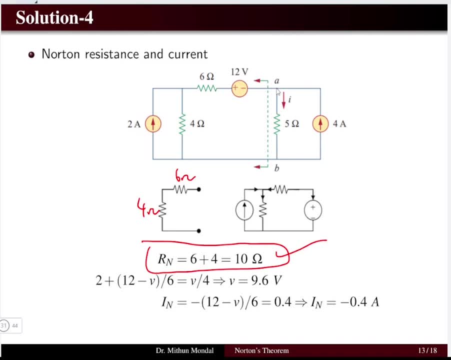 find the I Norton, what I am going to do, the load register. I will be short circuiting, So this part is short circuited, And then what I can do is that I can make the things to be simple by applying some source transformation and then I can determine the. 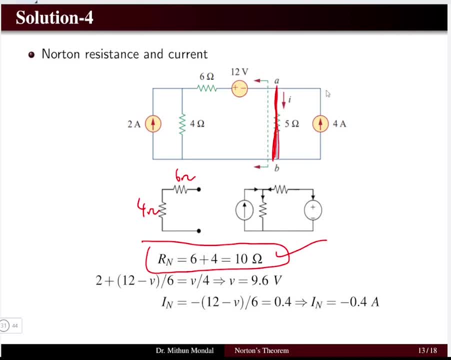 short circuit current. Okay, So if I am sorting this, this current source will always be sorted. So we will be having, like this, one circuit where we have the 2 ohm register, 2 ohm current source. we have We have 4 ohm current source. We have 4 ohm current source. We have 4 ohm current source. 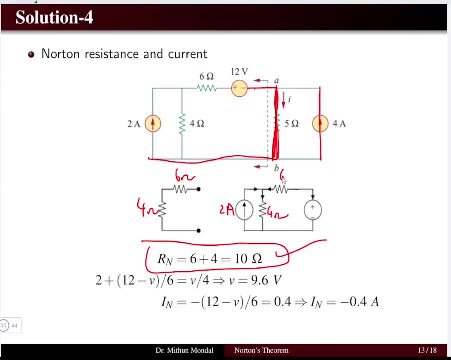 We have 4 ohm's current register, We have a 6 ohm register and we have a 12 volt voltage source. So this is the new circuit, that we have got it. So can we determine what is the current Norton current that is flowing? So these you can apply the KCL to determine the voltage here. What is? 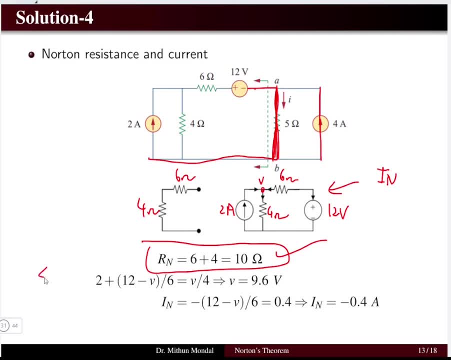 the voltage at this particular node. So you can apply the summation, all the current which is meeting and the particular node, that we have it and V is equal to zero, We can find the potential of that node that is 9.6 volt. This is in accordance with. 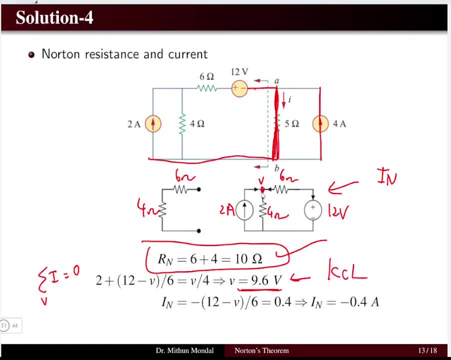 Kirchhoff's current law. Now, once we have obtained the voltage here, I can find that what is the current which is flowing this side? because that is the Norton current. Whatever the current is flowing this side, that is basically the Norton current. So, Norton current, I am getting as minus. 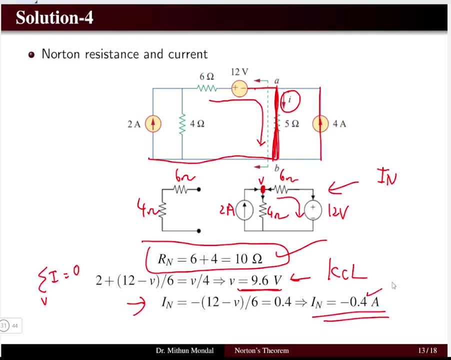 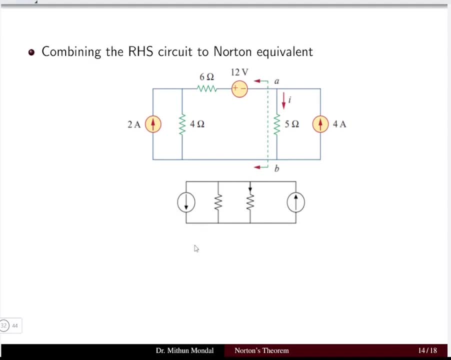 of 0.4 ampere. So I have got the Norton current and I have got the Norton register. So I have got the Norton resistance for this network. Now, once I got the value of Norton current and Norton resistance, I can reconnect the 5 ohm register, which was short circuited. 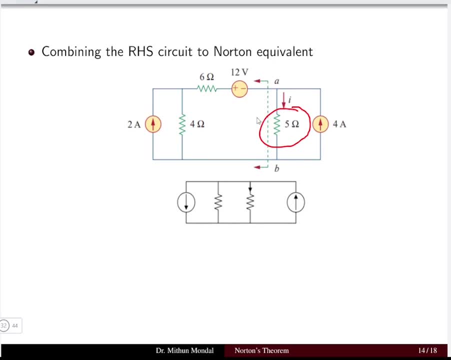 So we will be combining the remaining part of the circuit. So, since we were determining this side, so I have to connect these two part of the network that is the right hand side to the Norton equivalent circuit. So once I connect that I can determine what is the current which is flowing through the register. 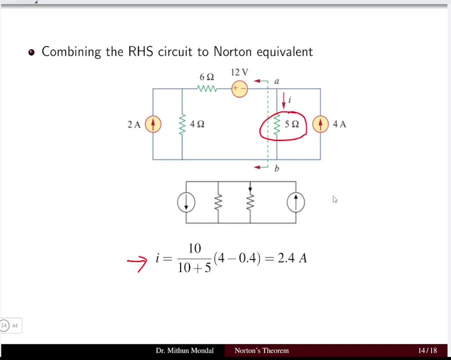 5 ohms. So that can be done by improving the circuit. So here you have 4 ampere, This one is 5 ohms, through which the current you need to determine, and then you can have the Norton current and the Norton resistance, which we have, the equivalent circuit So we can determine from. 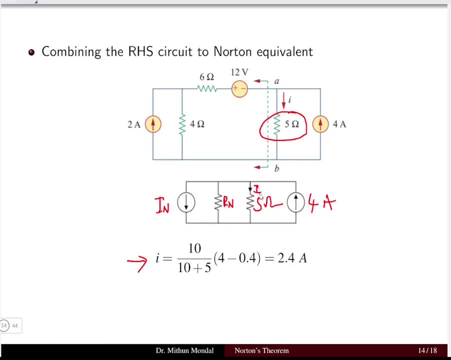 this circuit, what is the current which is flowing this side? So this is the Norton resistance Which is flowing here. So this current, you can apply the current division rule to apply that because we are having two resistances which are in parallel and two sources of the current which 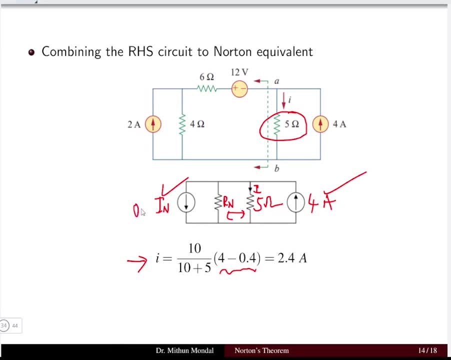 will be 4 minus 0.4, because the Norton current is 0.4 and we have a negative sign. so the direction is like this. So we can determine the current, that is, 2.4 ampere which is flowing through 5 ohm register. So in this way we can solve the problem using the Norton's theorem. 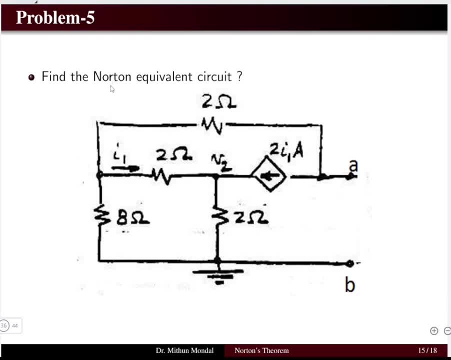 Okay, this is the final problem: Find the Norton equivalent circuit. Okay, so what is the difference in this problem? You have a current source that is 2 I1 and this is the dependent source. Okay, so we have one dependent source now. Now let us see how to do this type of problem, because we do. 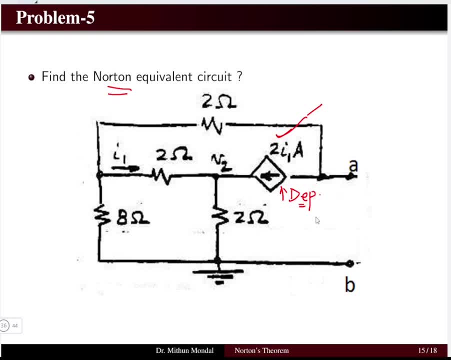 not have independent source in the circuit. We have dependent source in the circuit and, as I said, the value of R. Norton, you are not going to replace the value of the dependent source. It is only the independent source that has to be removed from the network. So how to do that in this problem? 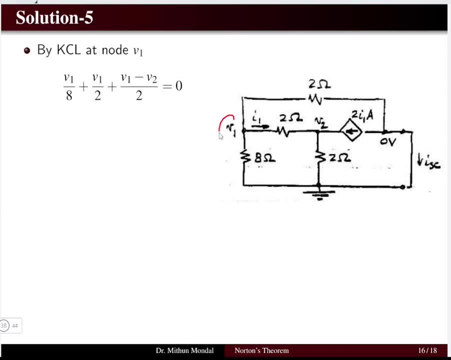 Okay so first we apply the Kirchhoff's current law at the two node V1 and V2 to determine the potential keeping the node to be sorted, because we need to find the Norton current, which is basically the short circuit current, At the terminal. Okay so here we have a dependent source and we can apply the KCL at node V1. This. 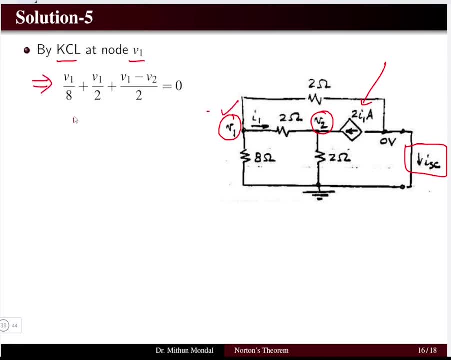 is the node V1.. We can write the KCL equation: algebraic sum of all the current to be 0 at the node V1.. So this is the KCL equation. KCL equation at node V2. we can write that algebraic sum of all. 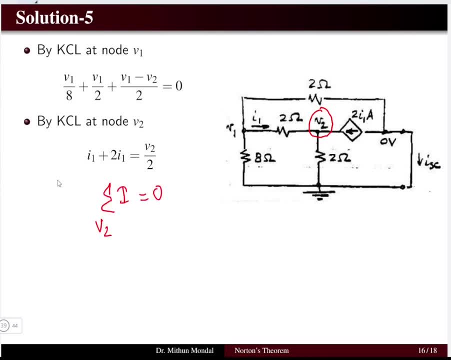 the current at the node V2 is equal to 0 in accordance with This equation. So all the current which is meeting and all the current which is leaving, that all current we have to add up to form the KCL equation. So I find that the V1 is my variable, V2 is the 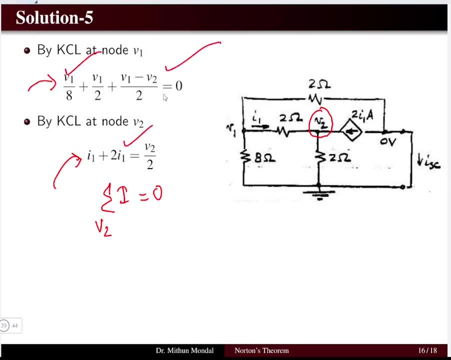 variable and I1 is the variable. Three variables in two equations. One more equation is there where the current I1 that is flowing, I can write V1 minus V2 by 2. So we have three equations and three variables that we need to find. So if we solve these three equations,